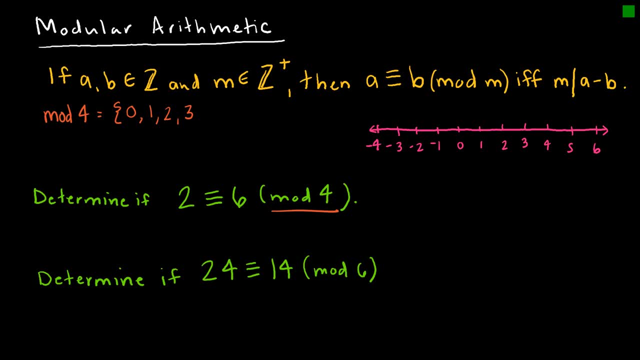 could get a remainder of 2, or I could get a remainder of 1.. And if I take something and I divide it by 4, I could possibly get a remainder of 1 or I could get a remainder of 3. now, if I got a remainder of 4, that would really be the. 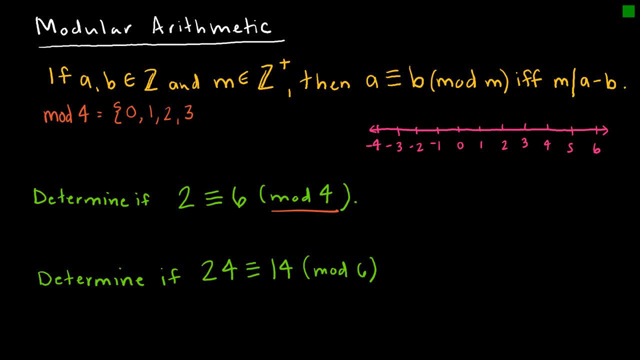 same thing as a remainder of 0, because 4 would be divisible by 4. exactly when means a remainder of 0? so these are really my only options, because we always like to look at the the smallest values. so now, if I'm looking at mod 4 and 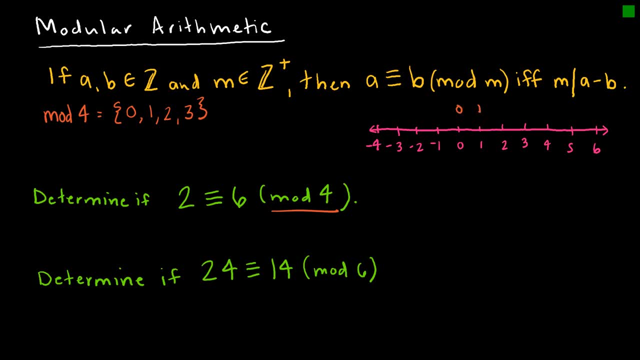 looking at my number line I've drawn, this would be 0, 1, 2, 3, just as we normally would think so on a number line. but with mod 4 the value of 4, 4 divided by 4 is a nice even number that has a remainder of 0, and 5 divided by 4 has a. 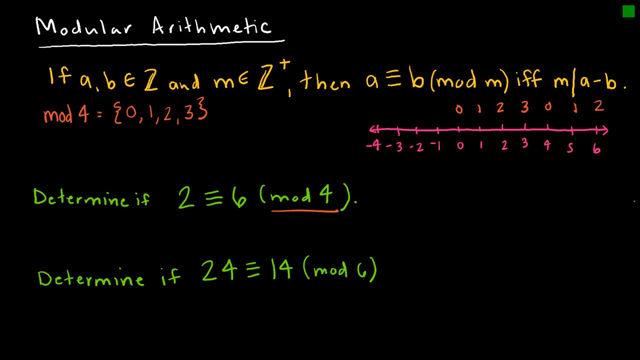 remainder of 1, and 6 divided by 4 has a remainder of 2, and similarly we could go in the opposite direction, where negative 1 would actually be negative 4 divided by 4, with a remainder of 3 and then 2, and then 1 and then 0, etc. so we can see what the pattern is is basically. 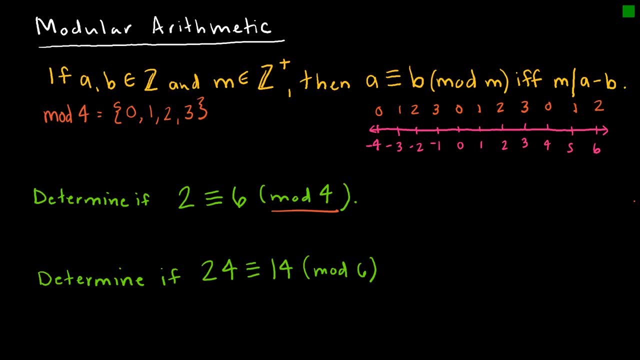 just 0, 1, 2, 3, 0, 1, 2, 3, 0, 1 2, 3, etc. so what we're looking for in our first example asks us: is 2 congruent to 6 in the world of mod 4? so looking at mod 4, 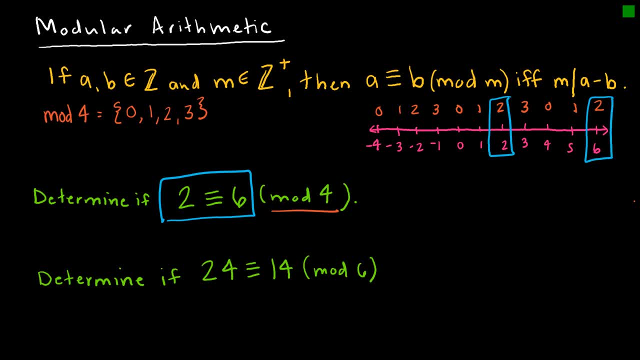 you can see that mod 4 has a remainder of 3 and then 2 and then 1 and then 0, etc. so, looking at mod 4, 2 and 6, if you'll notice both are 2, which means if I take 2 divided by 4 or 6 divided by 4, my 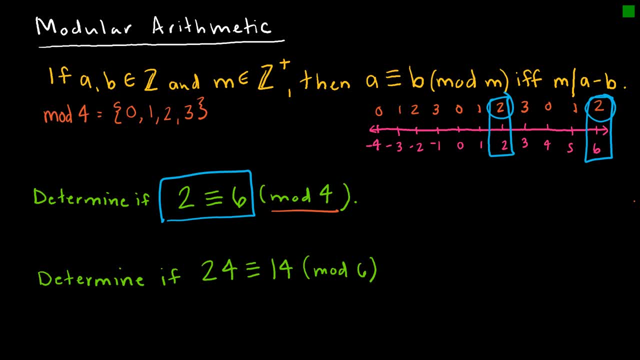 remainder is 2. exactly the same. so that's good. so that means yes, they are equivalent. now what I want to do instead is look at my definition. and my definition says I can determine that without making a number line and counting everything out by saying: is the difference between these two values? 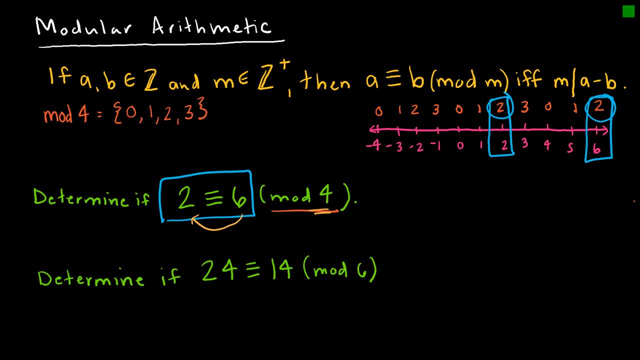 divisible by 4, and that is what we're asking here. so we're saying: does 4 divide 2 minus 6 or 6 minus 2 would give us the same result. so does 4 divide negative 4 and 4 does divide negative 4, and therefore we know that yes, 2 is. 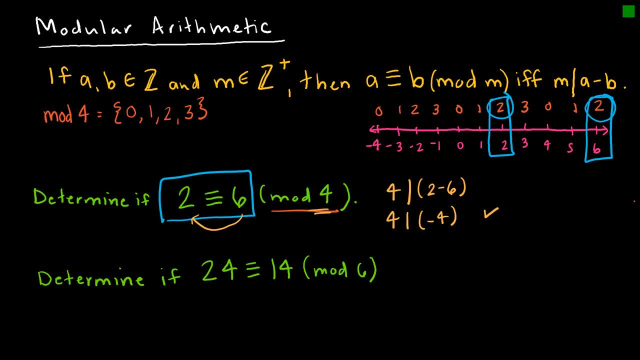 is congruent to six. So we're not saying that two is divisible by four or that six is divisible by four, but that these two are equivalent because they're the differences in their remainders is divisible by four. So let's look at our next one: 24 is 24 congruent to 14 mod six. So again, 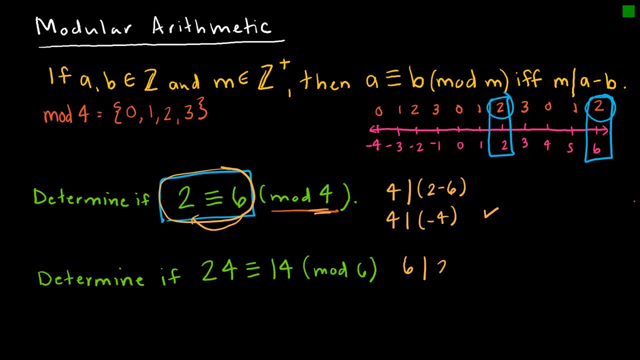 we're asking: does six divide 24 minus 14?? Does six divide 10?? And in this case, six does not divide 10 evenly, and therefore no, these are not equivalent. Again, we could draw out a number line. 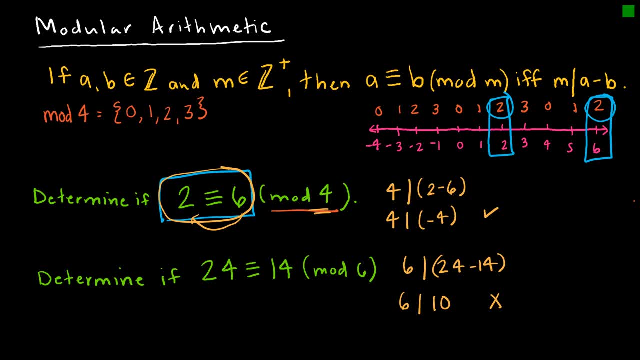 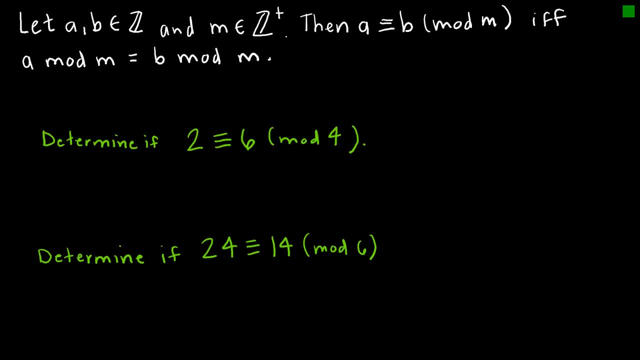 and we could see that visually. but hopefully you get the basic idea of modular arithmetic. We've just looked at the definition of modular arithmetic and I want to look at a theorem that really follows from that and I feel like this theorem is pretty straightforward, Essentially. 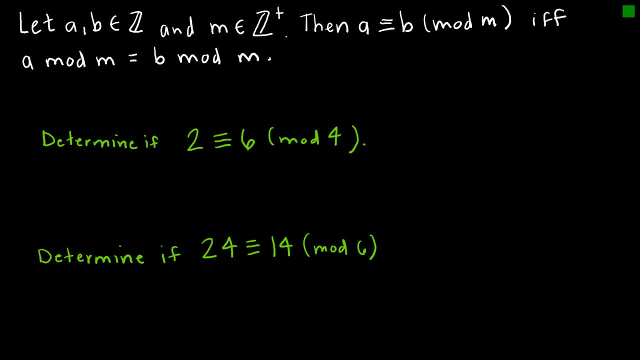 it's saying all the same things we had before: a mean integers, m is a positive integer, then a is congruent to b mod m, if and only if, and then a mod m is equal to b mod m. So really all we're. 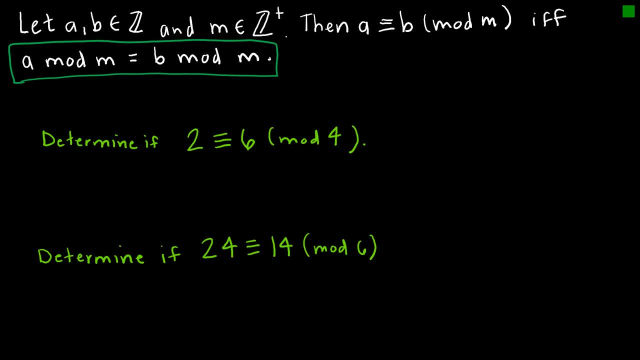 saying is: if the remainders are equal to one another, then they are congruent, and that's what we talked about when we looked at our last slide. But let's kind of look at it in terms of the mathematics. So I put the same two examples that 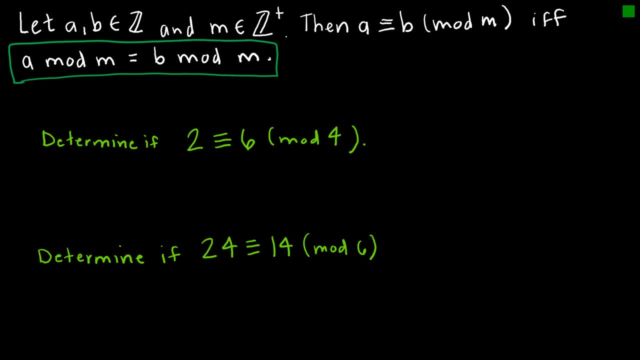 we had on the last slide and I just want to look at it in terms of when we looked at the division algorithm. So if I'm looking at two, I'm saying: does four divide two? And again we know the way that we can write this. We're saying: four times some number plus some number equals two. That's. 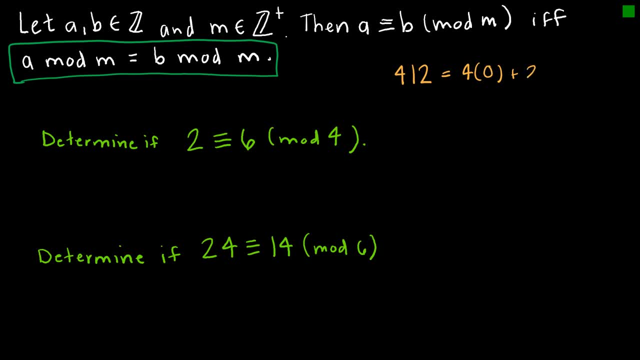 what we want to look for In this case. four times zero plus two does equal two. And then if I were going to write that in terms of r, which is the remainder, the remainder is equal to two mod four. So two mod four, So. 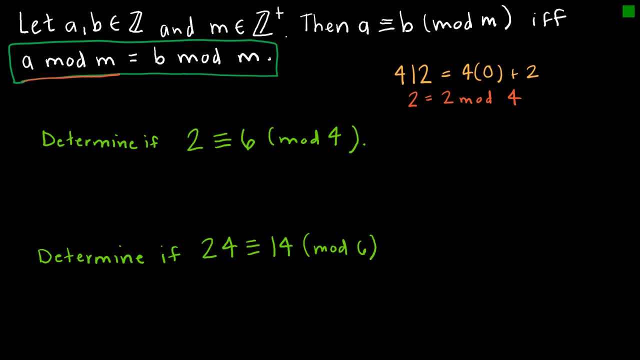 notice what I'm building up to here. a mod m- I'm saying two- is equal to two mod four. Let's look at six. So does two divide six? Sorry, Let me try that again. Does four divide six? I got confused for a minute And so again the way that we would write that is four times some number. 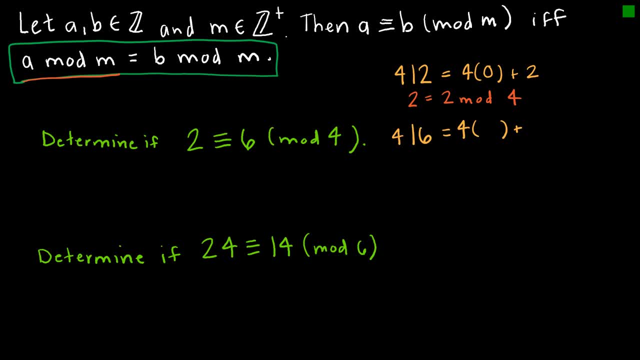 plus some number, using the definition of division, And in this case we would say: four times one is four plus two is six. So that's again, the remainder of two would be equal to six mod four. And so, notice, what I've just shown you is that, yes, in fact we already knew these were equivalent, But now I'm just showing you in another way that two is equal to two mod four, Two is equal to six mod four, And therefore two mod four is equal to six mod four. So that's again, the remainder of two would be equal to six. 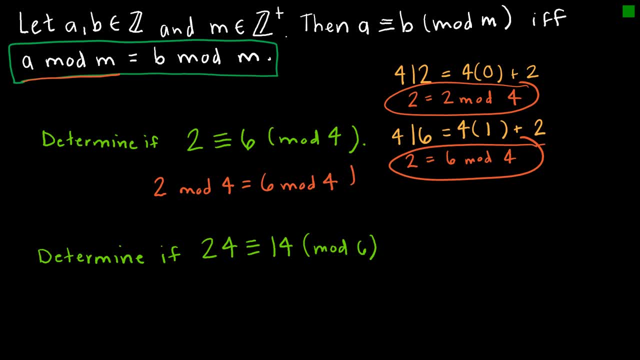 to 6 mod 4 and therefore we can say, yes, this is true. Let's look at our other example and again, we previously showed that this was not congruent. so let's take a look at how we might show that mathematically. So we're saying: does 6 divide 24? and if we take 6 divided by 24, we're saying: 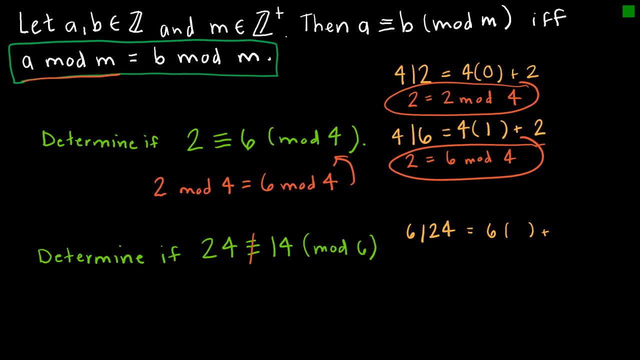 6 times some number plus some number is equal to 24.. In this case, 6 times 4 is 24 plus 0. So how would I write that? I would say that my remainder of 0 is equal to 24 mod 6.. 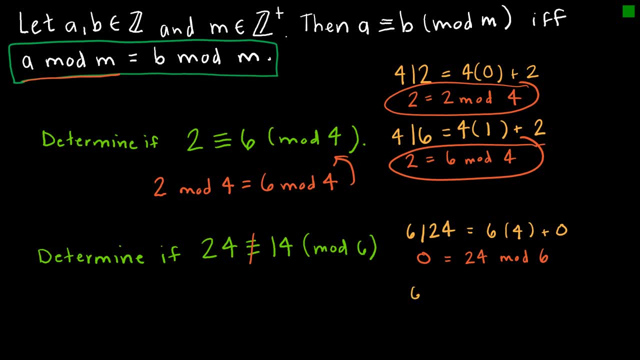 And now let's look at the other one. We have 14, so does 6 divide 14? and again we're saying 6 times some number plus some other number. This one would be: 6 times 2 is 12 plus 2 is 14 and notice here, my remainder is 2.. So 2 equals 14 mod 6 and obviously these values 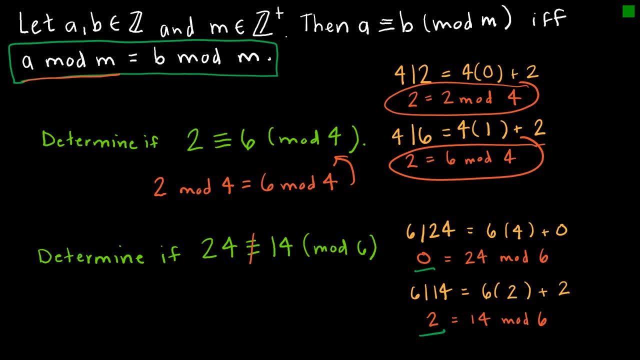 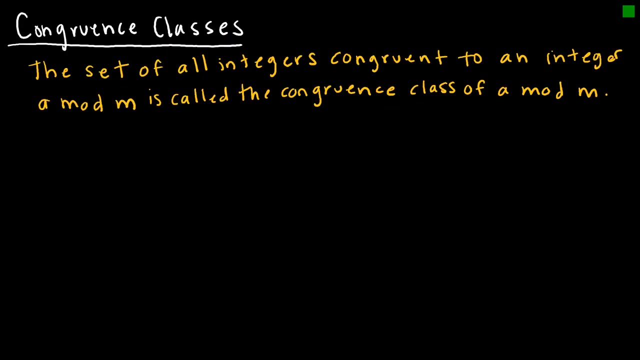 are not equal. Therefore 24 mod 6 does not equal 14 mod 6, and therefore we can say again that 24 is not congruent to 14 mod 6.. So we've sort of skated around this a little bit, but I really want to sort of define it for us. 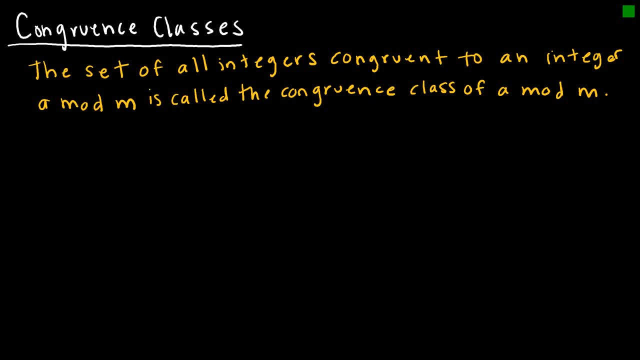 We're going to look at congruence classes, which are really just equivalence classes. So these are the same as equivalence classes and essentially we're saying that let's use mod 3 as an example. just because it's easy and there's less writing, I know in mod 3 that my remainder could be 0,, 1, or 2. And so for 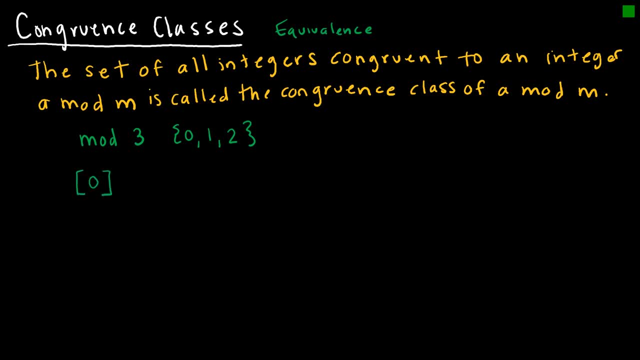 mod 3, I'm looking at an equivalence class for 0 and 1 for 1 and 1 for 2.. And what I want to do is just look at what values would be inside of there. And so if I'm dividing by 3, I know values like negative 6 are divisible by 3, and negative 3 are divisible by 3, and 0, and 3, and 6, etc. etc. etc. 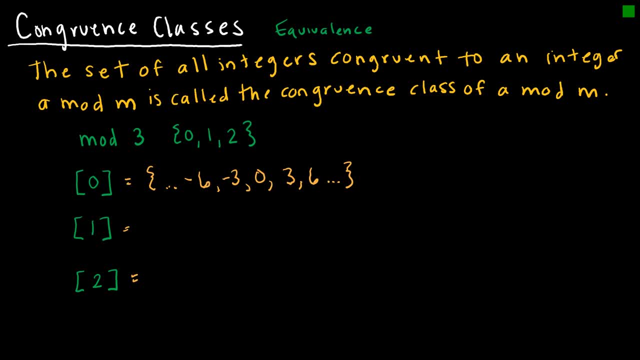 So what I can see here is that these are all obviously divisible by 3.. Now, looking at my next one, this is saying which values, when I divide by 3, would give me a remainder of 1.. So if I divided, say, negative 5, that would actually be negative 6 plus 1, so a remainder of 1.. 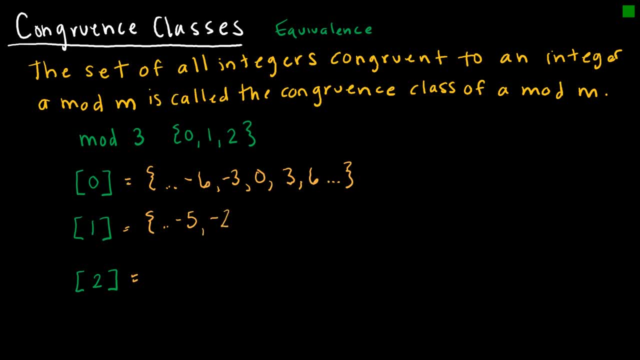 And then an answer of 2. An answer of sorry negative. 2. An answer of positive. An answer of negative: 1. An answer of 4.. So 4 divided by 3 would give me a remainder of 1.. 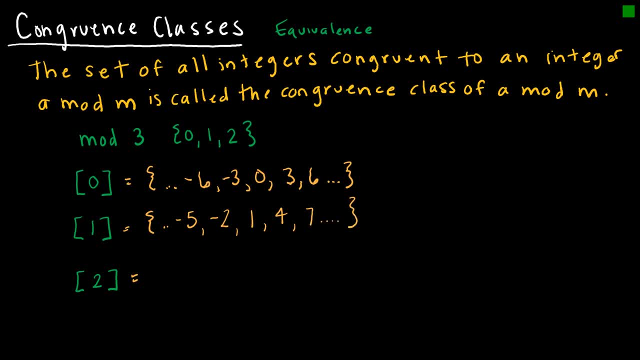 And we get the idea. And that goes on forever. And then, of course, if I look at the equivalence class for 2,, then I'm looking at negative 4, and negative 1, and 2, and 5,, etc, etc, etc, and we get the idea. 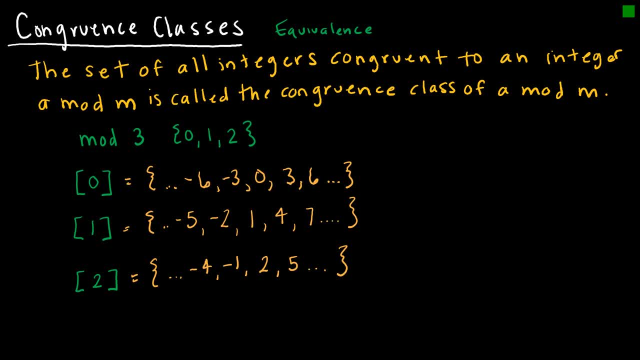 So a couple of things to understand with equivalence classes. First, if I took the union of all of these, then I should get the set of integers which makes sense. Basically. we're saying: all of these, all of the integers are included in 0 and 1 and 2 equivalence class. 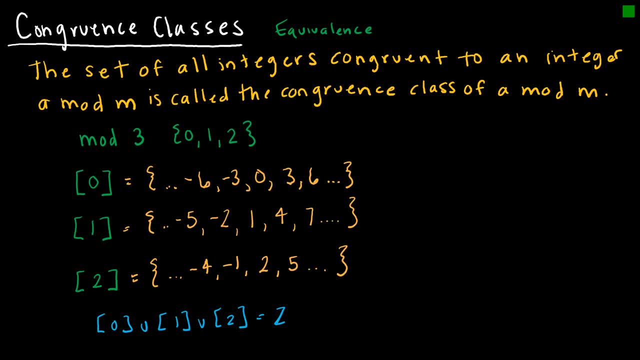 The other thing I want to look at is Going back to the way that we're writing our division algorithm. before, So we were looking at a equals dq plus r, and that's the way we were writing it before. So let's take a look at say 6.. 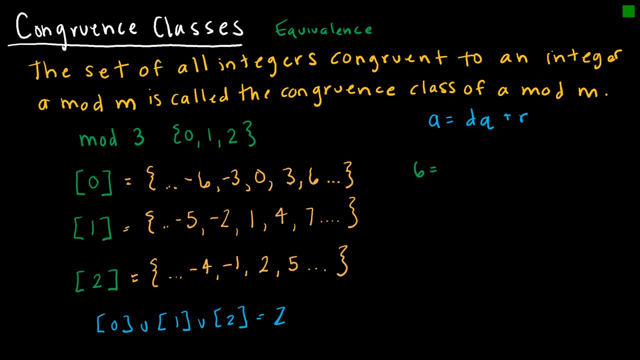 So 6 is equal to 3 times some number plus r, And, And in this case it would be 3 times 2 plus a remainder of 0.. Let's look at 1.. I'll choose a number from 1.. 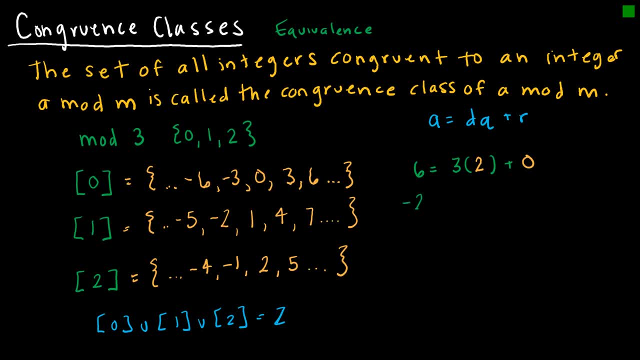 Let's look at say negative 2, just to be difficult, Negative 2 equals 3 times some number plus some number, And so if I took 3 times, in this case, negative 1. That would give me negative 3.. 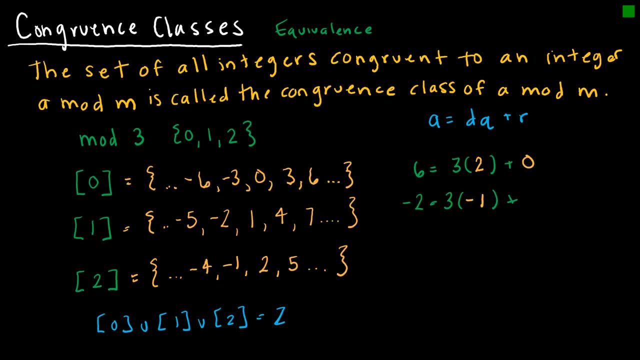 And then I would have to then add 1 to get negative 2. And I could do that for any of the values inside that equivalence class. And then if I look at, say, some value from 2, let's look at 5.. 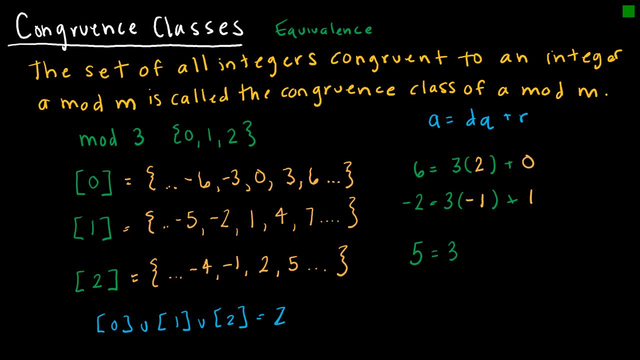 So if I look at 5, then I'm saying 3 times some number plus some number, And 3 times 1 would be 3 plus 2 is 5.. And what I want you to notice is that the 0 is the remainder. 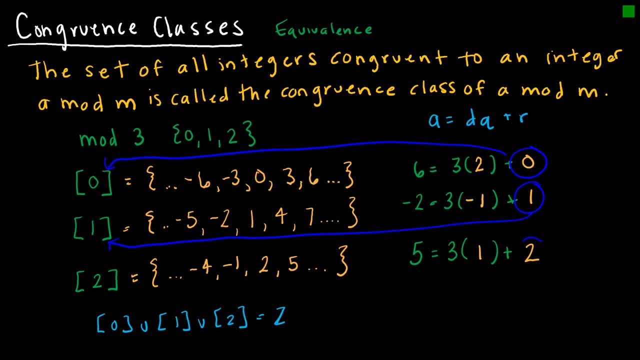 And that corresponds to the equivalence class And of course the quotient, in this case the q, I'm sorry, the d. the divisor is whatever. our modulo is, So mod 3.. We're obviously dividing by 3.. 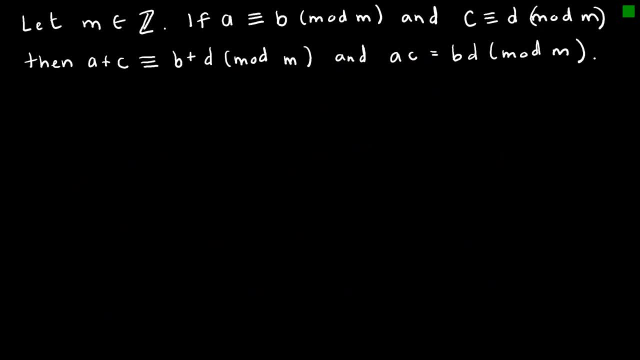 So what we're leading up to here is to be able to actually do some calculations in modular arithmetic. But before we do that, I want to look at an extension of the modular arithmetic definition with you, Just to make sure we sort of understand as we move forward. 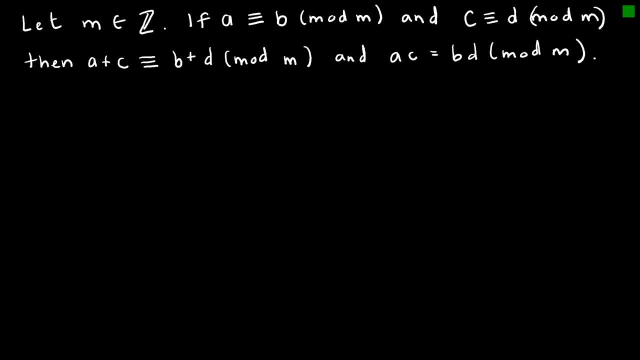 And I want to look at the proof with you. So again, let m be a, And this should say positive integer. I apologize, So let m be a positive integer If a is congruent to b mod m and c is congruent to d mod m. 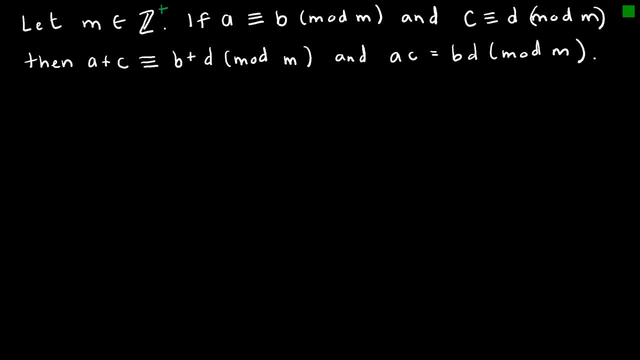 then a plus c is congruent to b plus d mod m, And a times c is equal to b times d mod m. So again, this is going to make sense because we're going to be looking at addition and multiplication in our upcoming lesson. 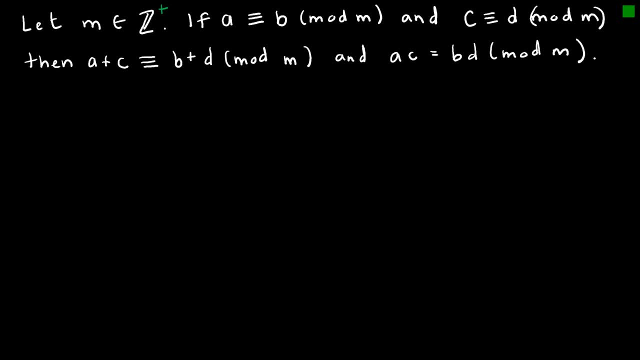 But let's go ahead and look at a proof. So, as we always do with proofs, we're going to lead a lot on definitions etc. So I can say: since a is congruent to b, mod m, And again I'm just going to be using the definition. 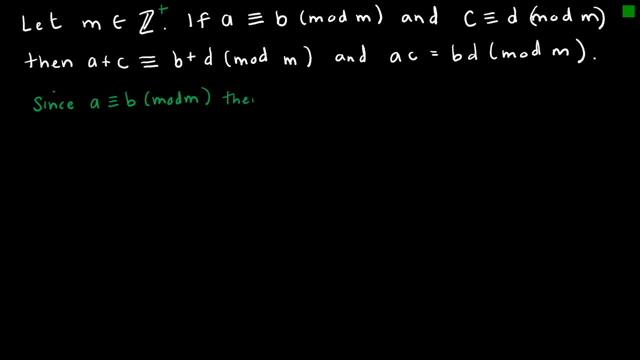 So a is congruent to b mod m. Then I can say that b is equal to a plus plus. We'll say k m. Where k is some integer? Oh, I'm having trouble today. So where k is some integer. 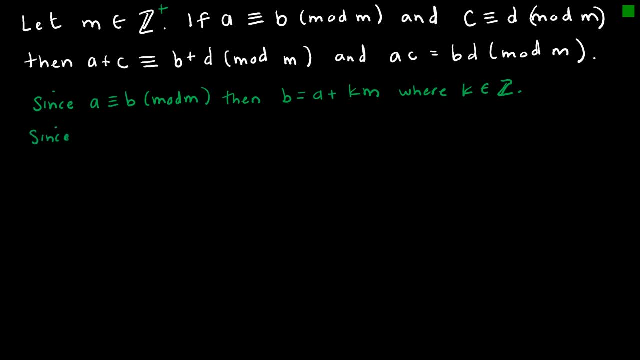 And similarly, since c is congruent to d, mod m, then I can do the exact same thing. I can say: d is equal to c, plus we'll say l m, Where l, of course, is an integer. 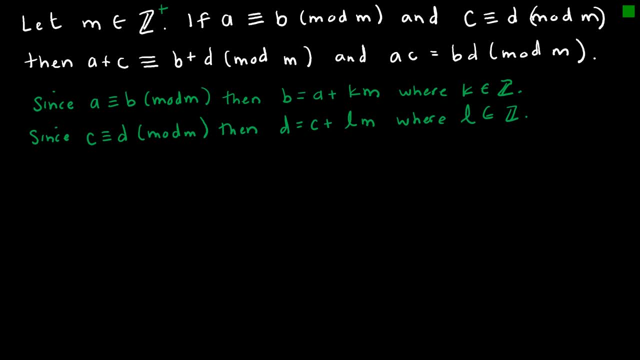 So essentially, I've just defined them using my division algorithm. that I did before. So now let's look at the proofs. Looking at the first one I'm looking at: a plus c is congruent to b plus d mod m. 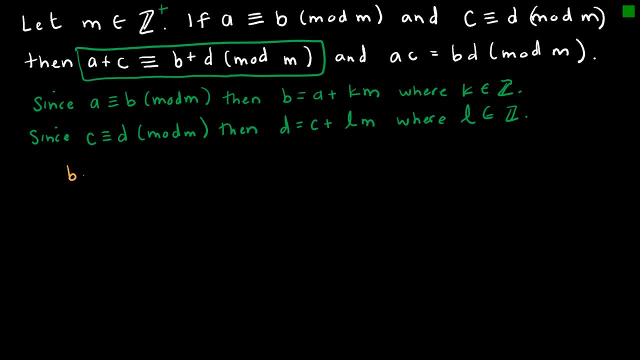 So I can say that b plus d. I should have outlined that in yellow to kind of keep everything straight. b plus d is equal to- and this is just substitution- a plus k, m plus c plus l, m, And then of course I'm going to do some simplification. 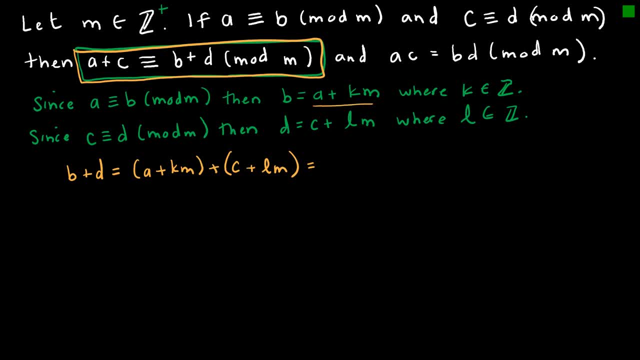 knowing that I want to end up looking. I'm going to do some simplification: knowing that I want to end up looking kind of like this, which is, of course, what the division algorithm tells us, And so I can say: this is a plus c plus k, m plus l m. 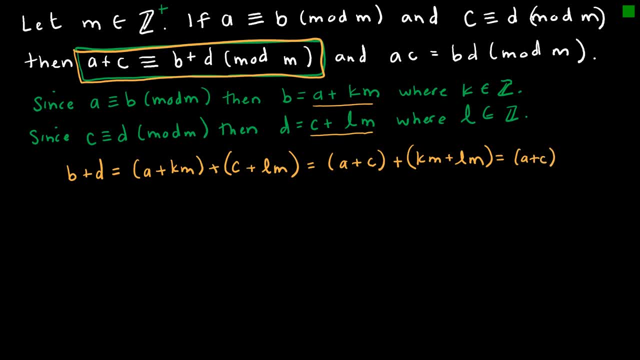 Or, even better, a plus c plus m, k plus l. And now you can see that I'm looking at the exact same format of how I'm going to divide, How we have written this before, So let's look at the other one. 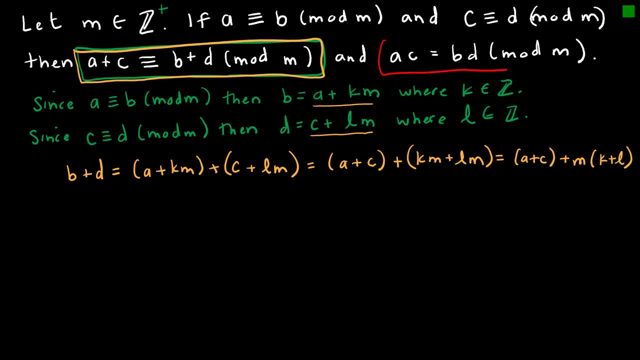 The other one says: a times c equals b times d mod m. So again I'm going to look at b times d, which is equal to a plus k m- I'm sorry, Yeah, c plus l m. So essentially I'm multiplying. 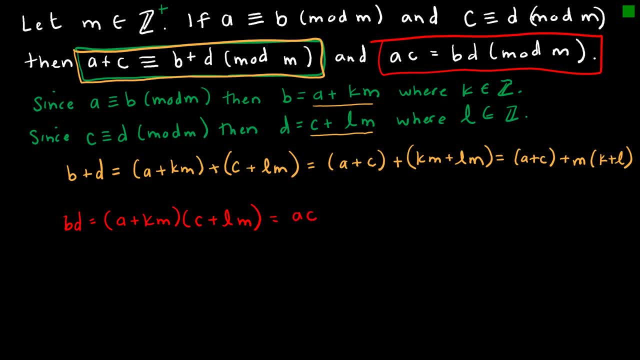 And then I'll FOIL that out. So I would get a c plus a l m plus k c m plus k l m squared, Which really what I want to look at is a c plus m And then Whatever inside. 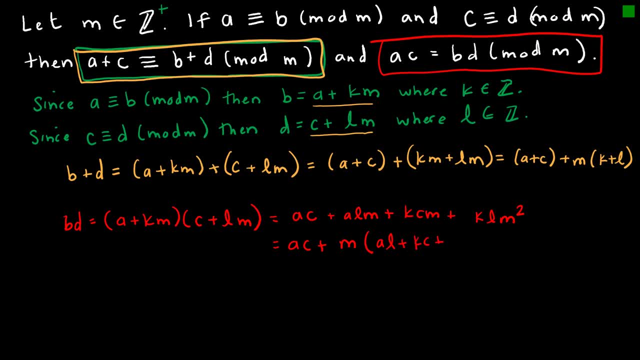 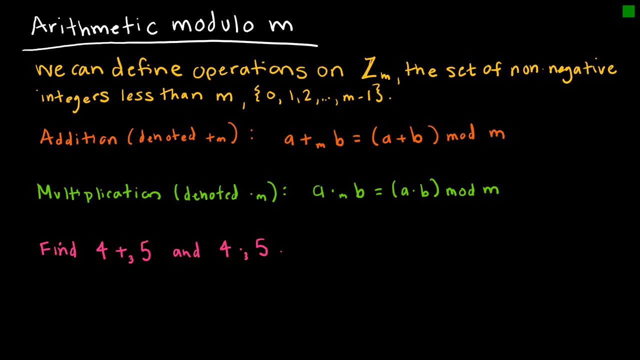 So in this case it would be a l plus k c plus k l- m, And again, because I'm able to write it in the correct format, then I have essentially proven that those are true. So now we're going to look at arithmetic mod m. 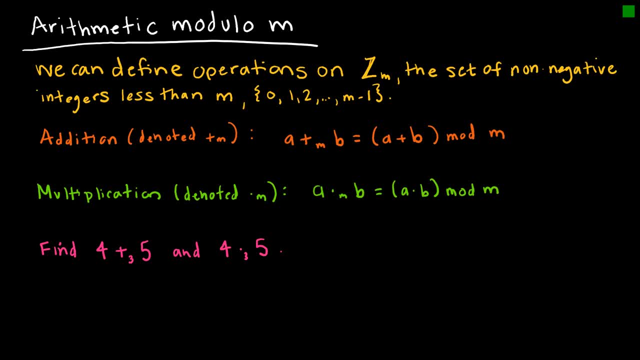 And, if you'll notice, this is exactly what we just proved prior to doing these examples. And so I'm looking at addition And at multiplication, Which essentially says that if I'm going to add two values, mod m, then I'm going to add the values as I normally do, and then determine the mod of those values. 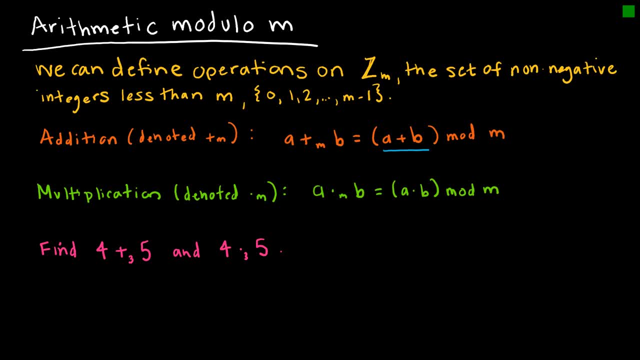 So for addition again, a plus m in mod m. Same thing for multiplication. If I'm taking a times b mod m, then I'm just going to take a times b and then determine the mod of that. So let's take a look at an example. 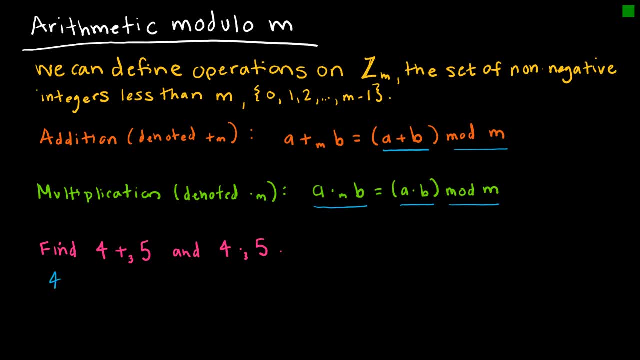 So this makes sense to us. If I'm looking at four plus five and this is mod three, This tells me to take four plus five mod three. So four plus five is nine And nine mod three. And remember, mod is just what is the remainder when you divide. 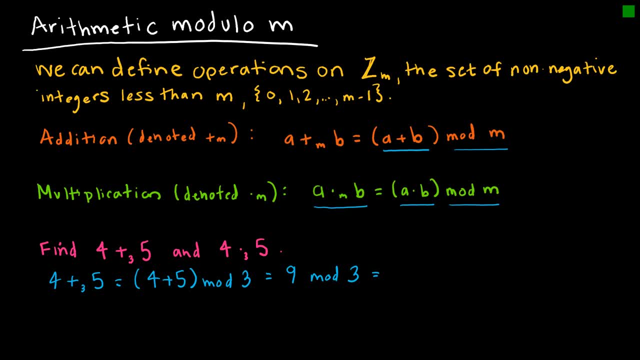 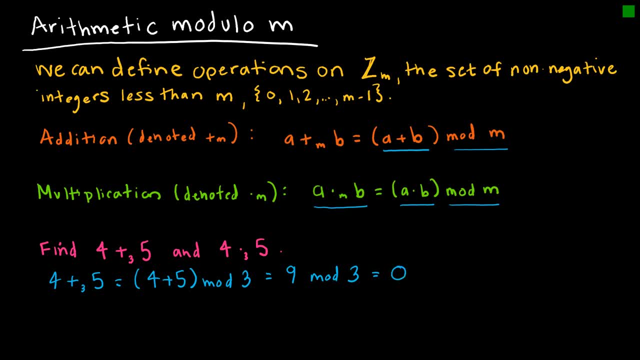 So my solution for that is zero. Let's look at multiplication Four times five mod three, And again four times five would give me, And again four times five would give me Four times five mod three. I just forgot to write it out. 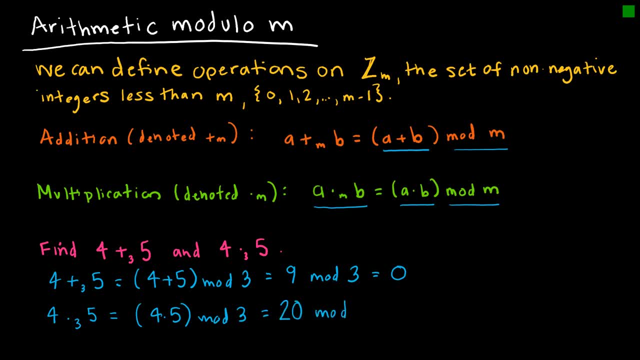 Four times five would give me 20 mod three. And remember, I'm looking at if I took 20 divided by three. and if I took 20 divided by three, I'm looking at if I took 20 divided by three, what would be my hair group? 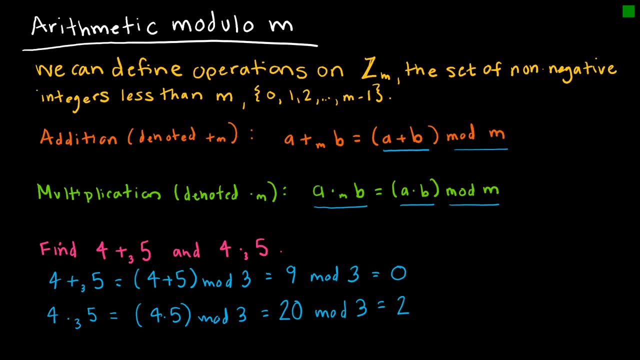 What would be my remainder? And my remainder would be 2..